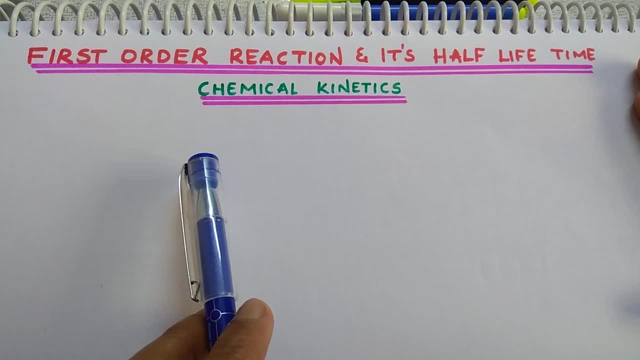 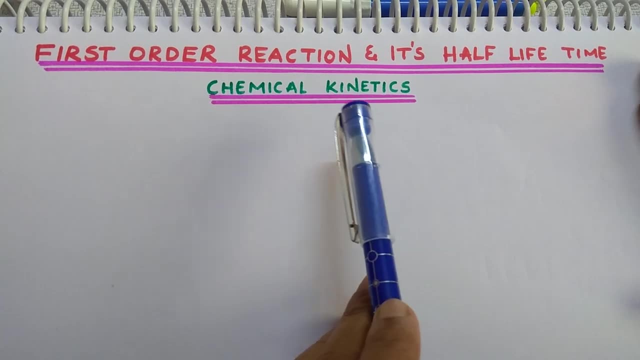 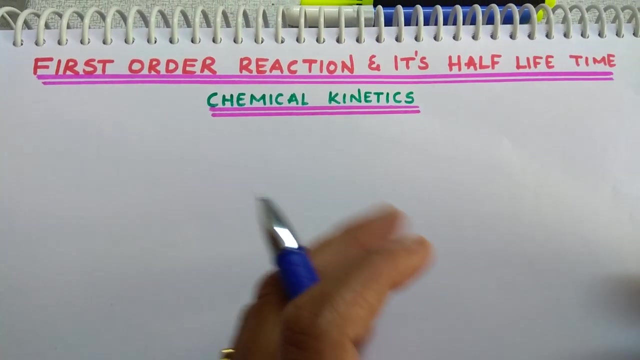 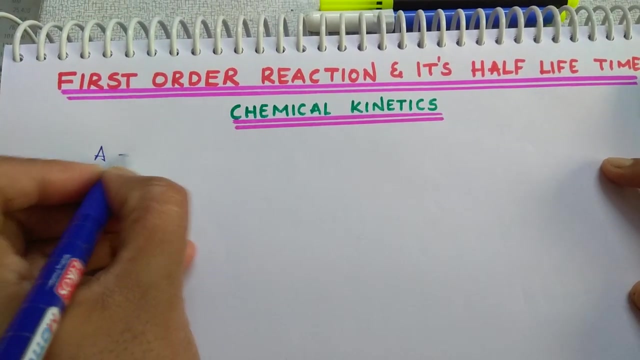 Hi students, in this session I am going to discuss derivation for rate constant of first order reaction and its half lifetime. This topic is from chemical kinetics, chapter First order reaction. we can say that rate of a reaction is depends upon the only one concentration of the reactants. For example, reactants A is converted into products B. 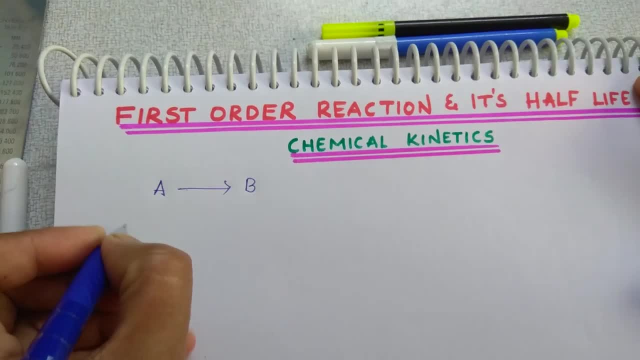 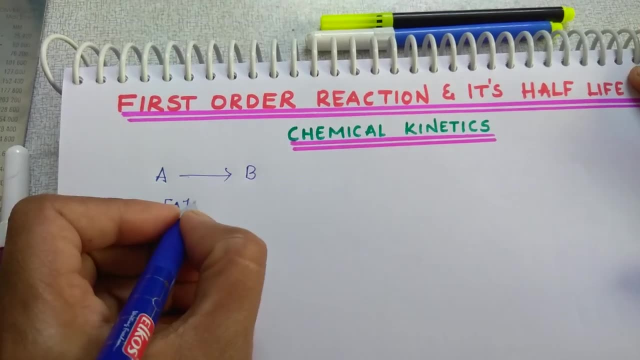 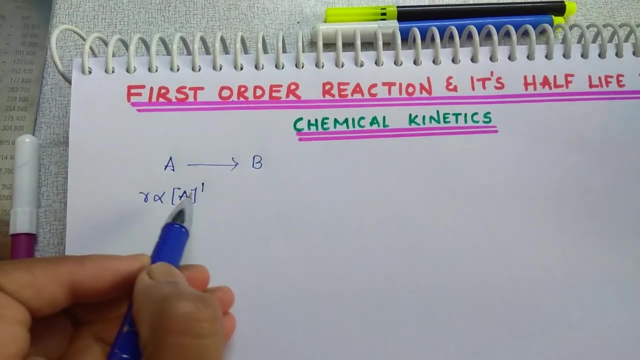 And, according to rate law, how to write a rate expression for this is: rate is proportional to concentration of reactants. And here we are telling: first order, so put 1.. Why I am keeping 1 here? Because it is in first order. If it is a 0 order, you can put 0. And rate. 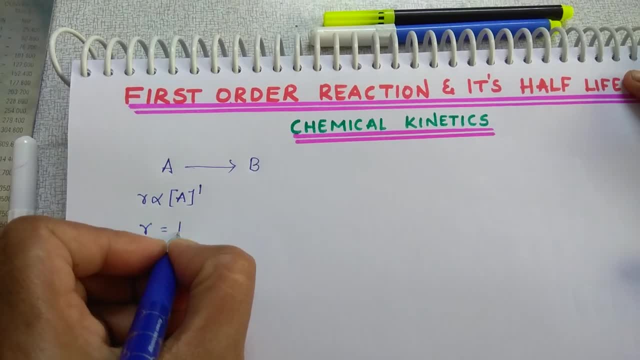 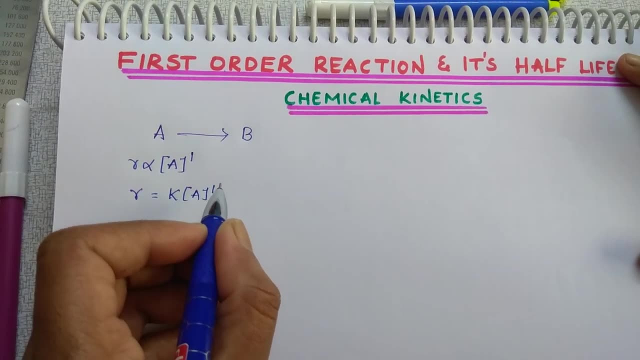 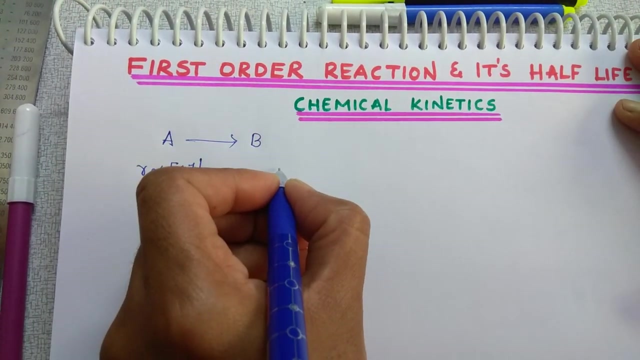 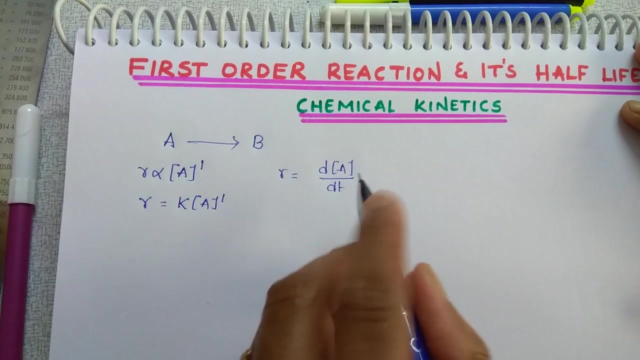 is equal. to remove this proportionality and put a constant k, Then we get the expression: rate is equal to k Into A, to the power of 1.. And according to the rate expression, how you can write rate expression is: see: rate is equal to D of A by DT concentration with respect to time. 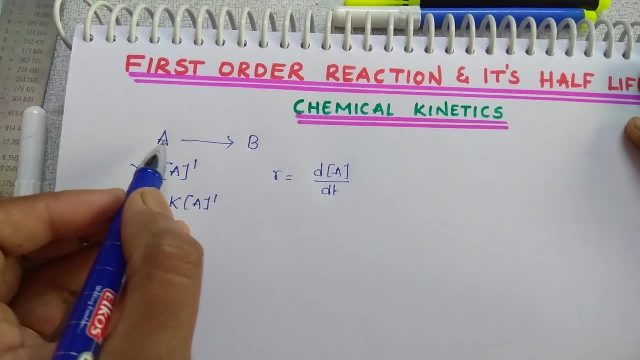 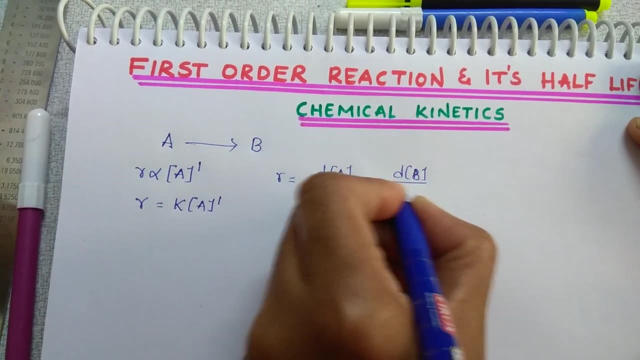 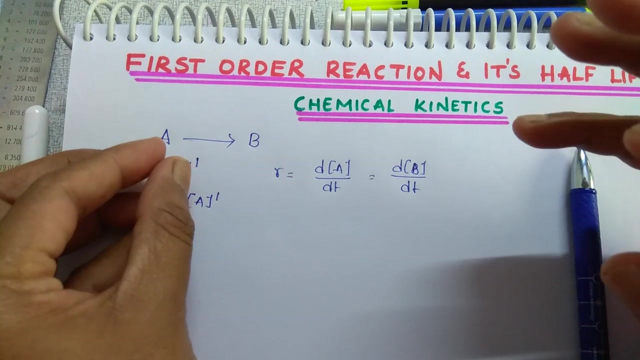 What is rate Concentration with respect to time? Here I wrote for reactants. Now I am going to write for products. Rate is equal to concentration of products with respect to time. But here, if you take initially 100 moles, after some time some amount of the reactants are converted. 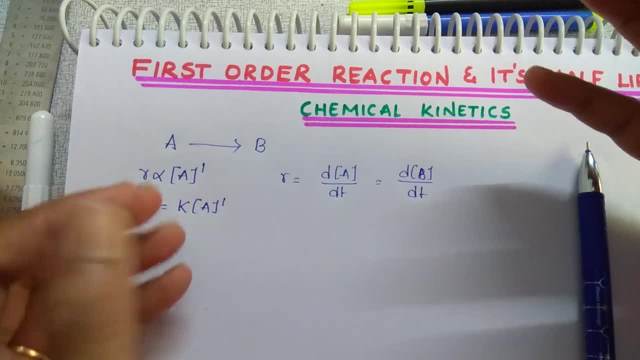 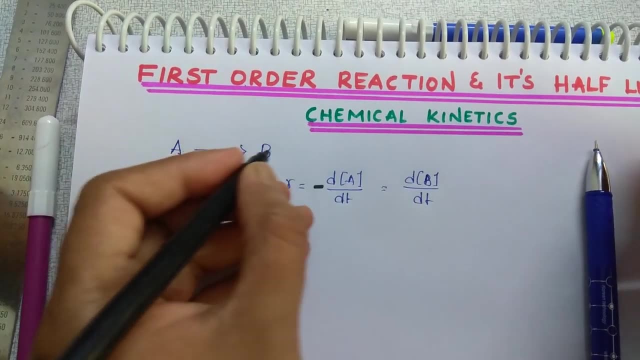 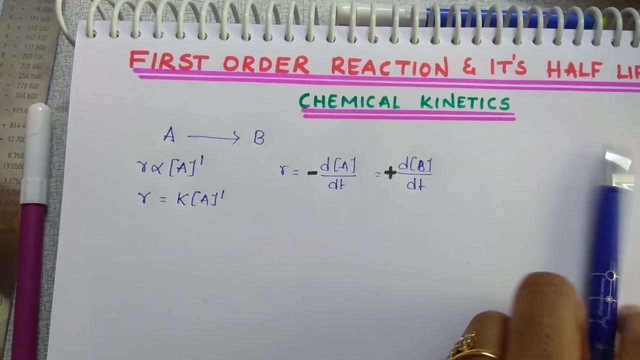 into products. So you can say that with respect to the time. along with the time, concentration of the reactants decreases, So I put minus before A, And products concentration increases with respect to time, So I put plus before concentration of B with respect to time Here. 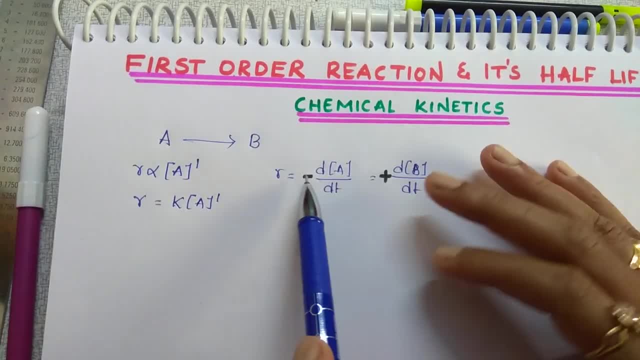 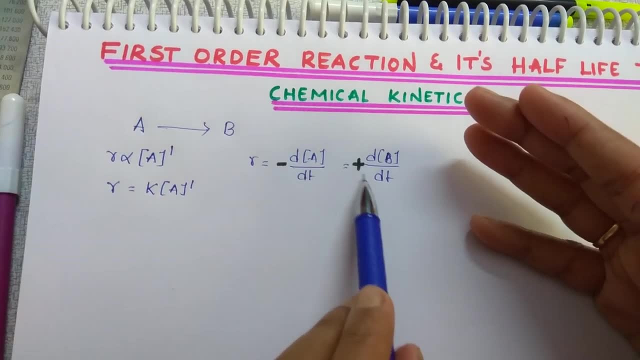 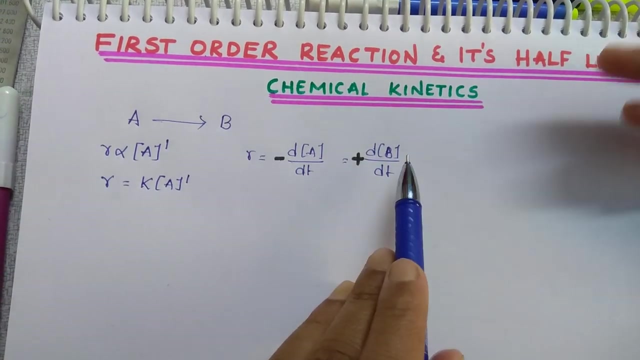 it doesn't mean that rate can be negative or positive. This minus and plus is not for this rate, Which actually indicates that concentration of reactants is decreasing here and here. positive indicates that concentration of products are increasing Here. concentration of reactants decreasing here, concentration of products increasing Now. this is also 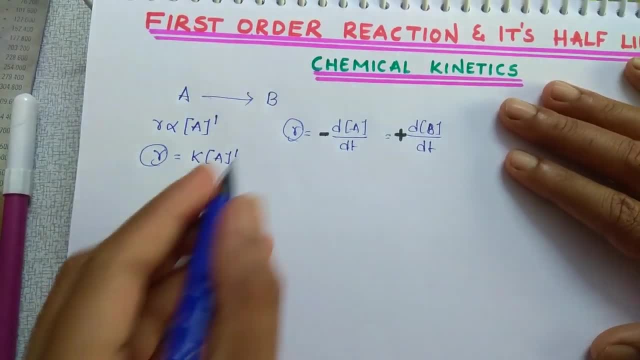 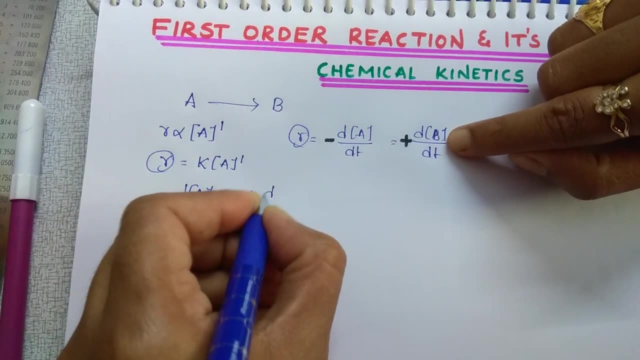 rate, and this is also rate. Now equate these two. What we get D of A by DT is equal to plus D of B by DT is equal to 2.5 times. Now let's take this again. We get: D of A by DT is equal to 2.5 times. 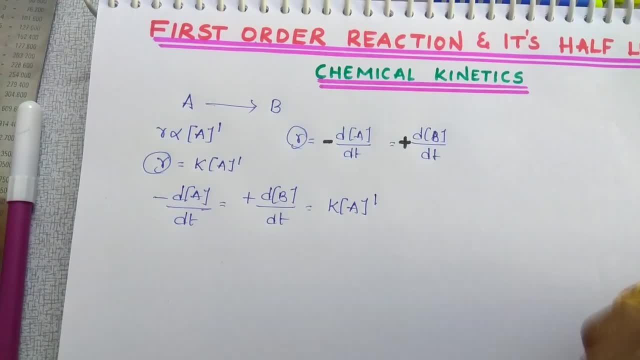 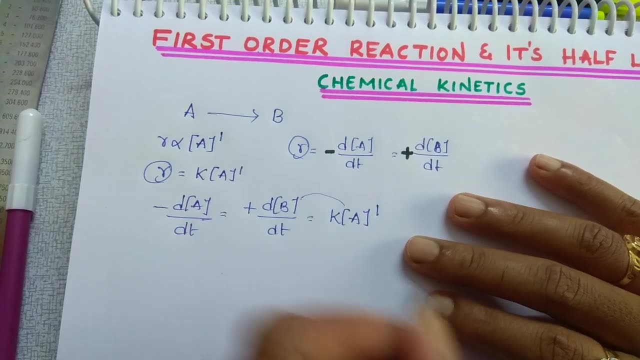 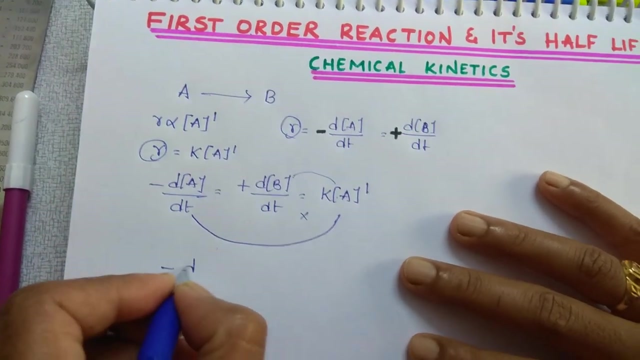 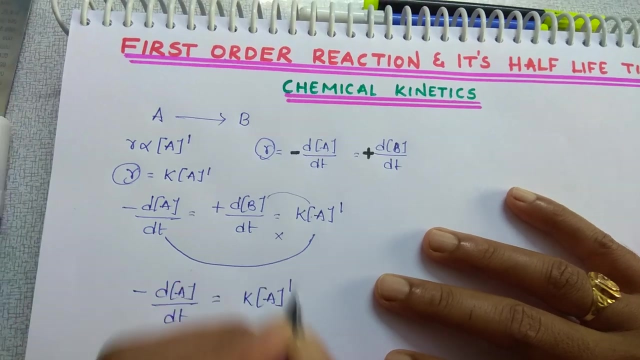 k into a to the power of 1. now, if you observe here, this is also a variable, this is also a variable. both are different, right? so you cannot do integration for these two. now take these two expression: same variable minus d of a by dt, which is equal to k, into a to the power of 1. 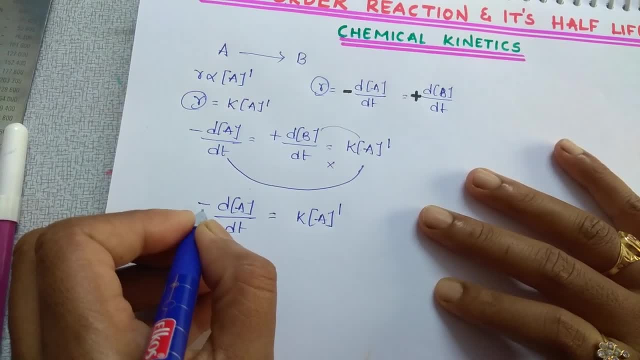 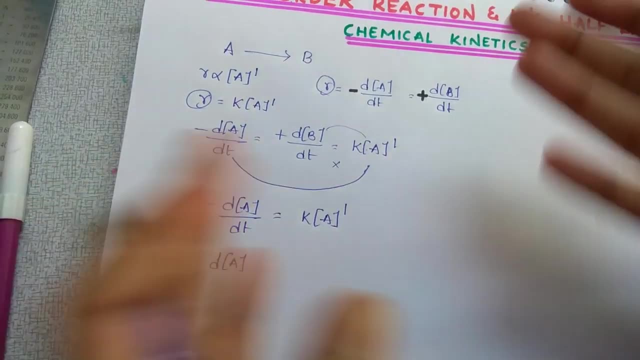 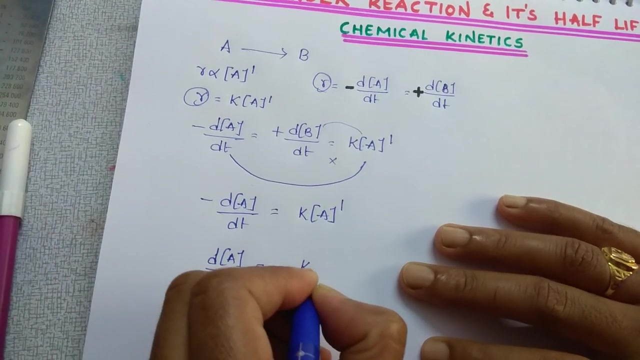 now what you do is just move this minus over here, and what you get for that, what you should do- multiply both the sides with minus, then you will get minus. minus becomes positive. d of a by dt is equal to minus k into a, to the power of 1, or simply a. you can write: 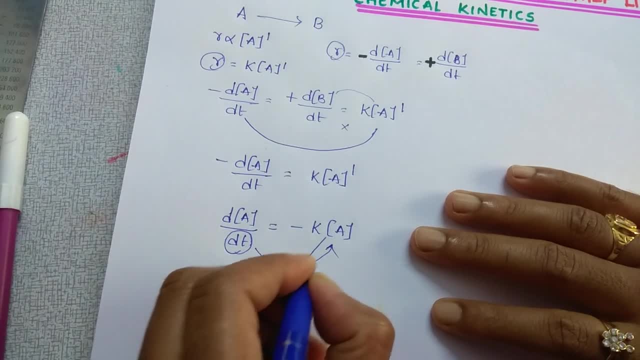 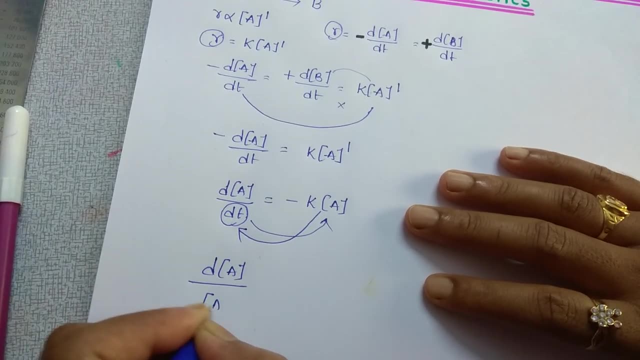 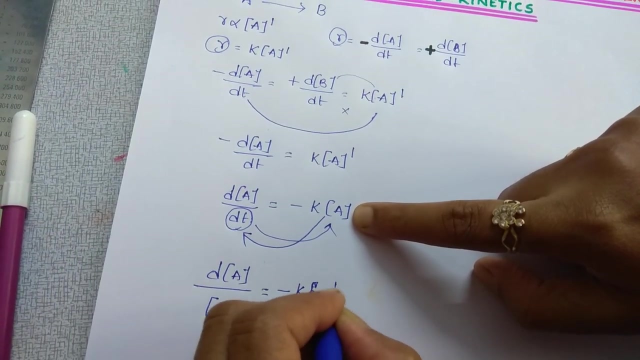 now move this dt term toward this side and concentration of a toward this side, then you get d of a by a, which is equal to this dt term. i am moving towards the right hand side, so we get k into dt. this is the expression we got now. do integration to this on both the sides. 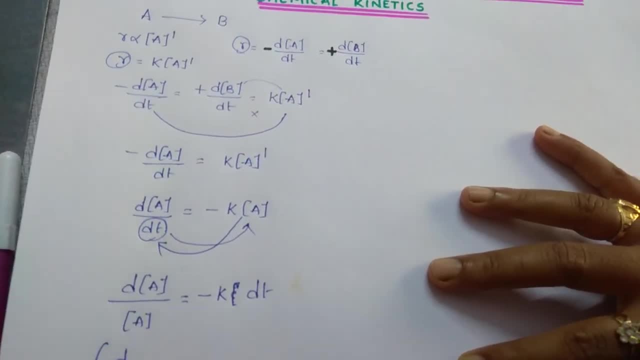 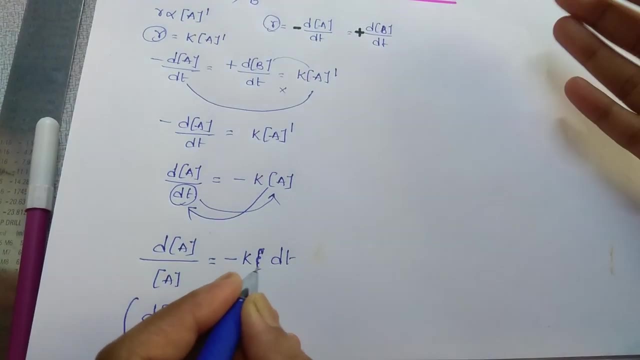 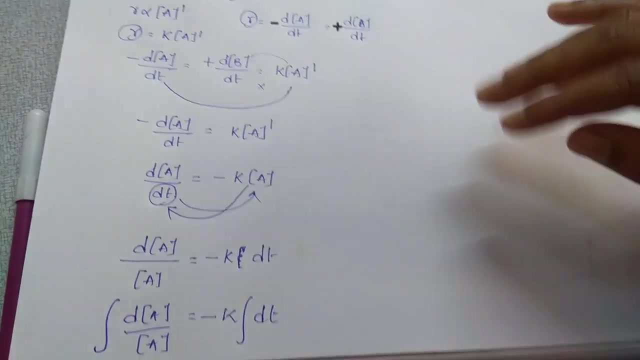 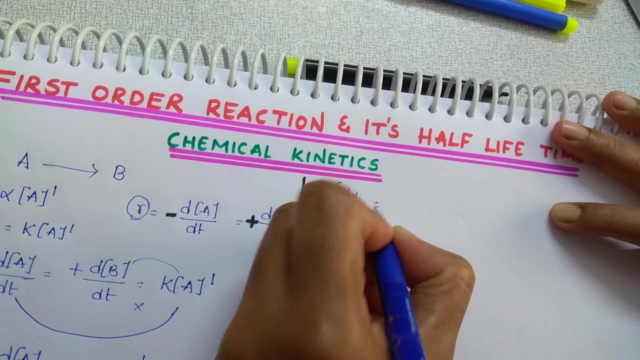 i am doing integration. integration d of a by a is equal to k, is in a constant. so a comes, k comes out. a, a, a, d, t is left. i will tell you two formulas. integration of d of x by x is equal to ln of x. integration of d of x is equal. 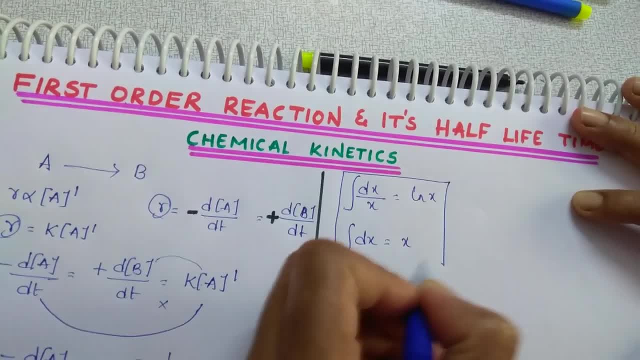 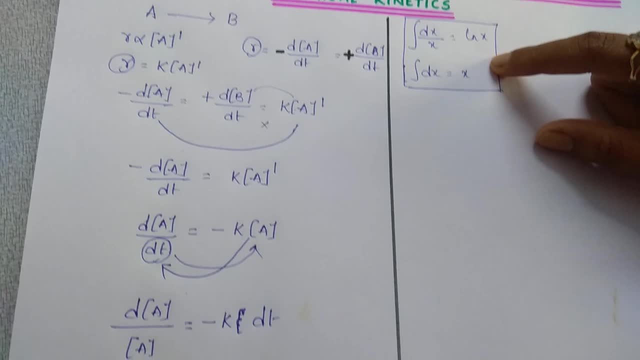 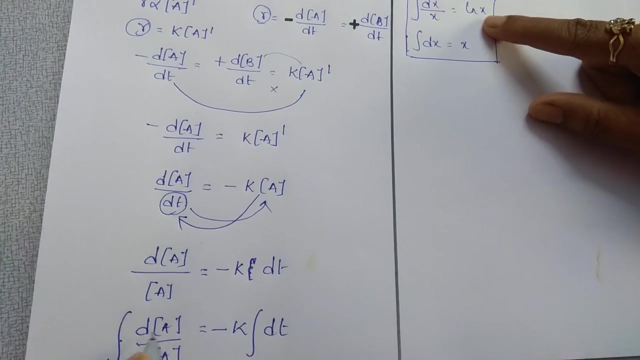 to x clear. these two formulas are enough to solve this integration, to do this integration. so what you get here, see here integration of integration of d of a by a, then you will get how much what you will get. students tell me this is like integration of d of x by x, then you will get ln of x. so here you. 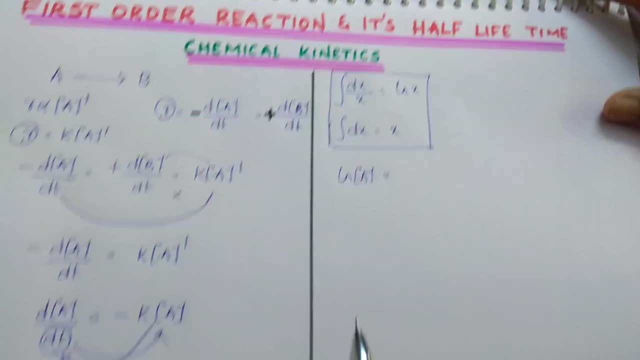 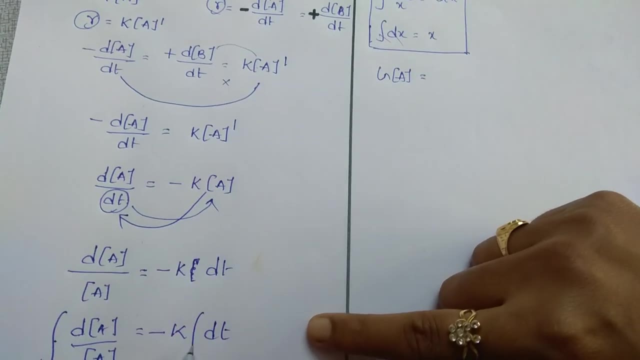 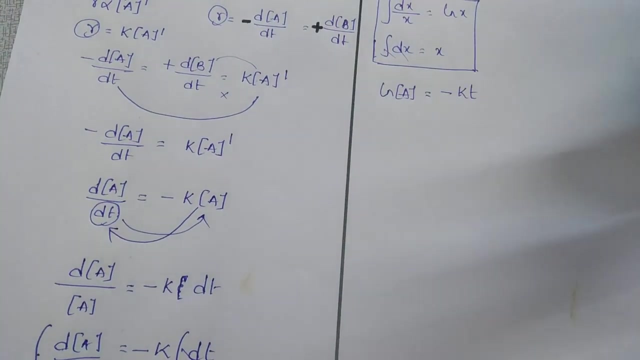 will get ln of a, which is equal to integration of d, of x is equal to integration. differentiation gets cancelled. you will get x, so here also it is on the same form. so you will get minus k into t, and whenever we are doing integration we get a constant called integration constant, i. so this: 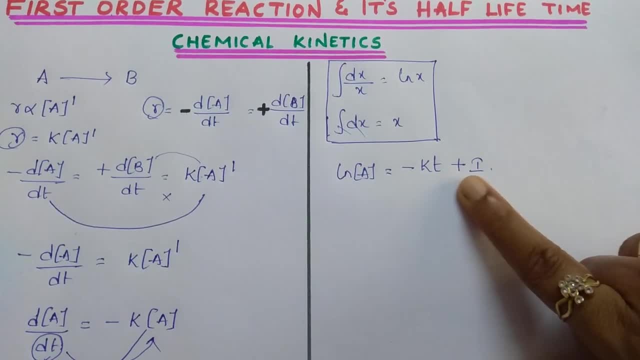 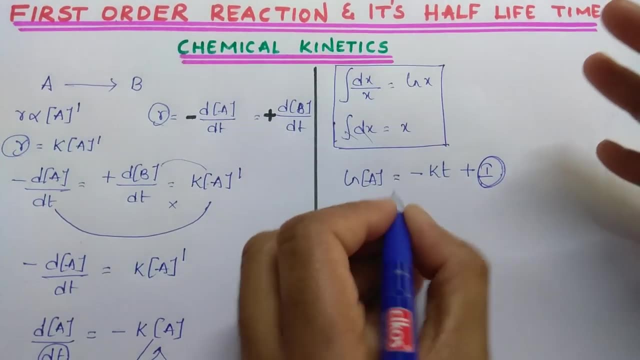 is the expression we got. what is this expression? ln of a is equal to minus kt plus i. how to find this integration constant? i value is: when reaction is not started, then time t is taken as zero because reaction is not started and whatever the total concentration is there that we take. 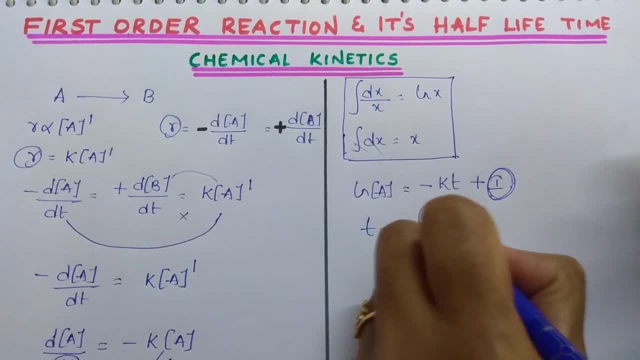 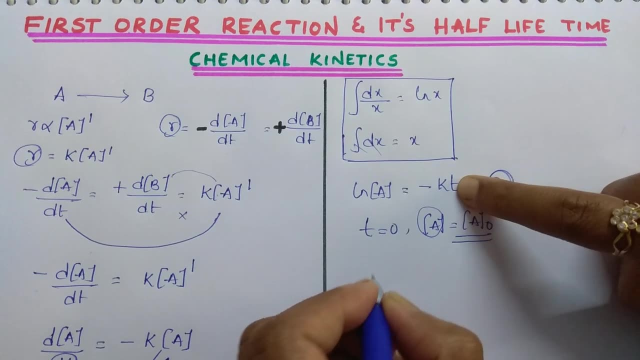 is initial concentration. so a becomes a naught because reaction is not started. and substitute these two values over here. t value zero. so here put zero, ln of a is equal to kt plus i. so this is the expression we got. what is this expression? ln of a is: 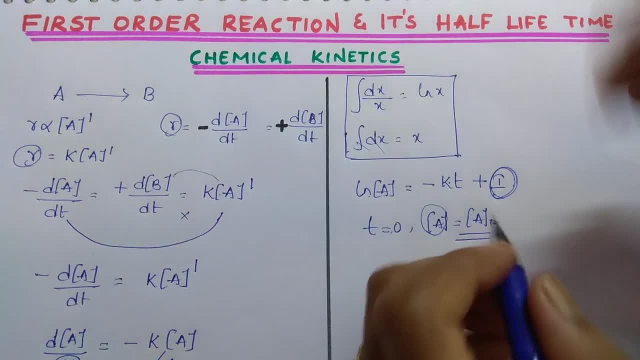 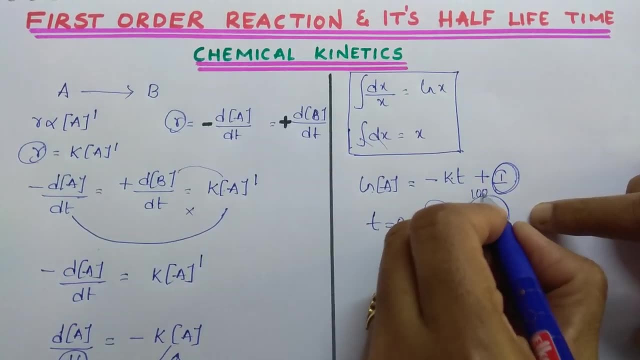 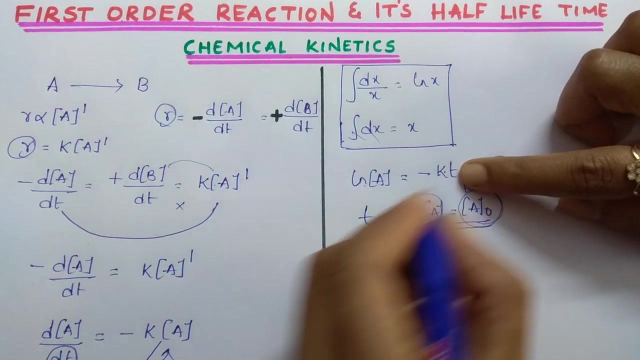 equal to ln of a becomes ln of a naught. why we are taking a naught? because reaction is not started started. so how suppose initially 100 moles is that 100? you have to take it now. ln of a naught, which is equal to minus k. into what is the t value students? zero plus i, then k into zero. 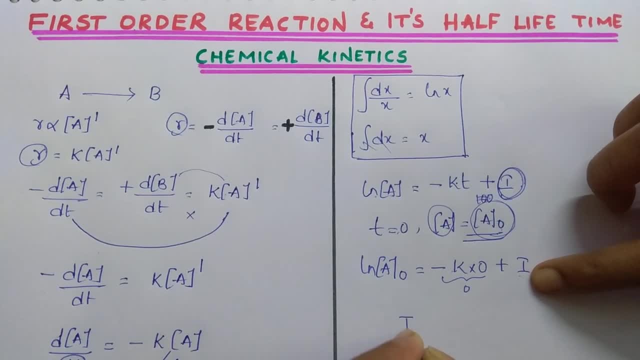 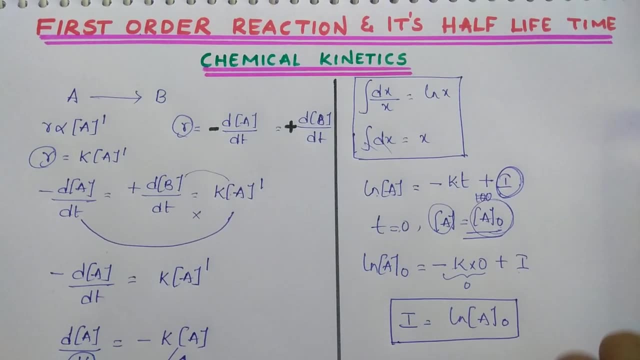 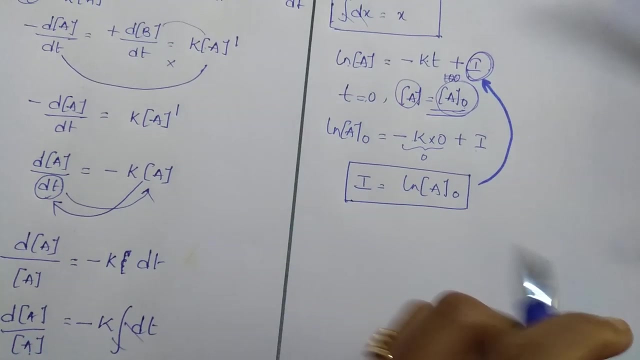 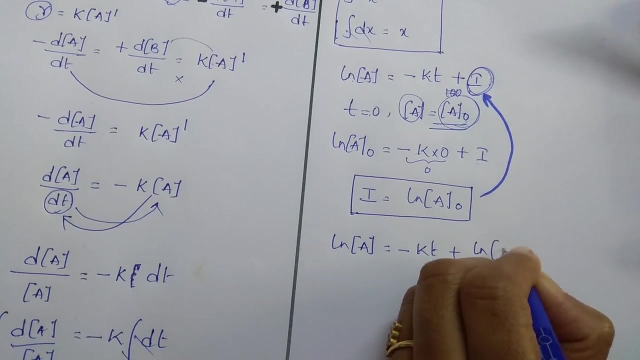 this term becomes zero, then i is equal to what ln of ln of a naught. now we got, i value this, i value. what you have to do is substitute here, substitute i value there. then what you get ln of a is equal to minus kt plus ln of a naught. now take this expression, suppose. 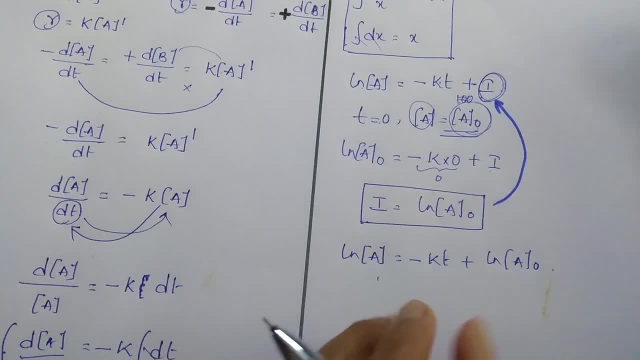 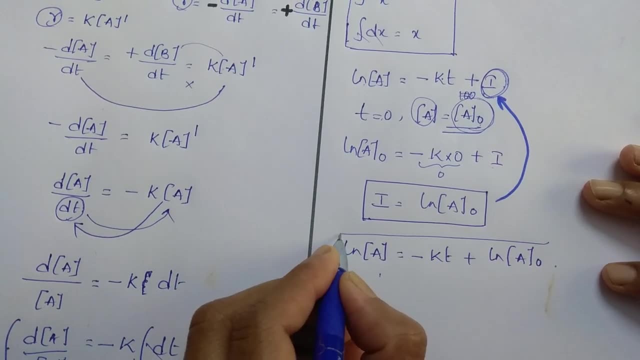 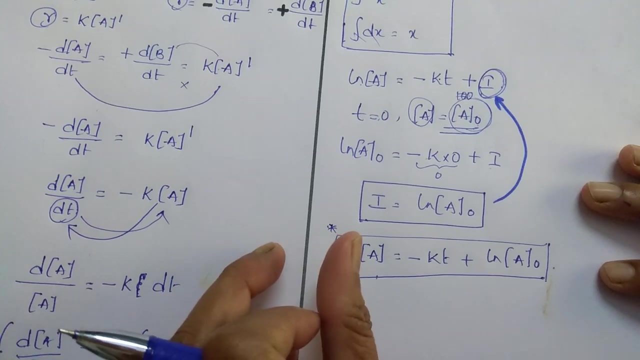 if you move this, i will draw the graph here, but it will create little confusion, so i'll draw the graphs later. 17. де 8.a. but this step is useful to draw the graph, so keep this step in mind. now move this kt towards the. 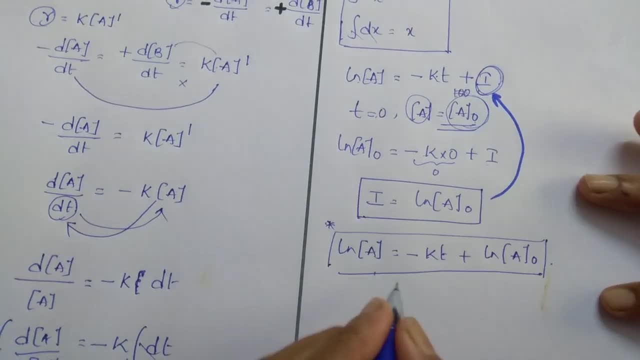 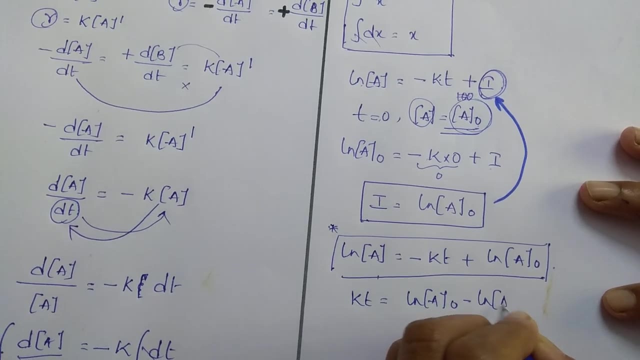 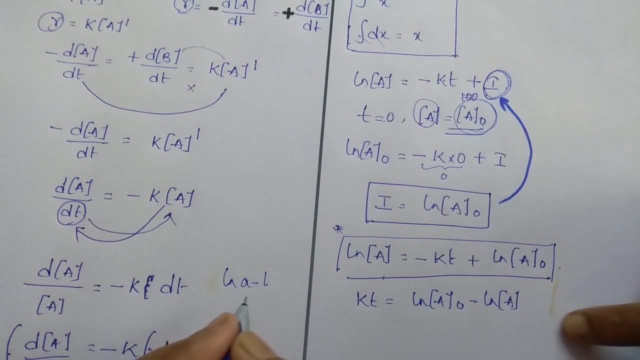 left hand side and move this ln of a term towards the right hand side, then we get kt is equal to ln of a naught minus, if it come this side, ln of a. then I will tell you one formula here: ln of a minus ln of b. so you have to add here one more formula also: ln of a minus ln of b is equal to: 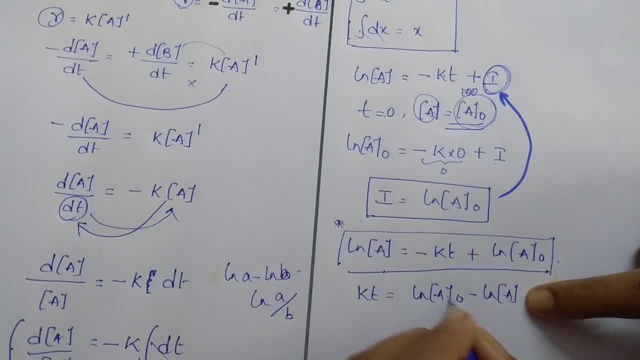 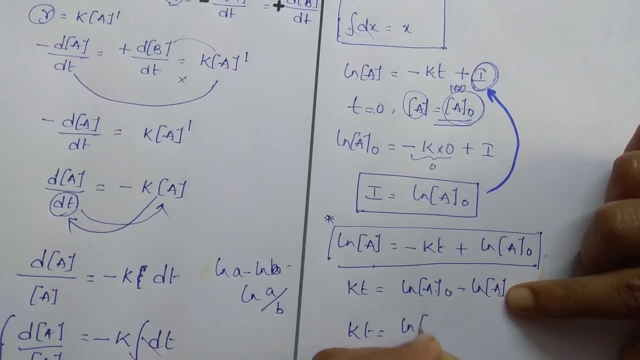 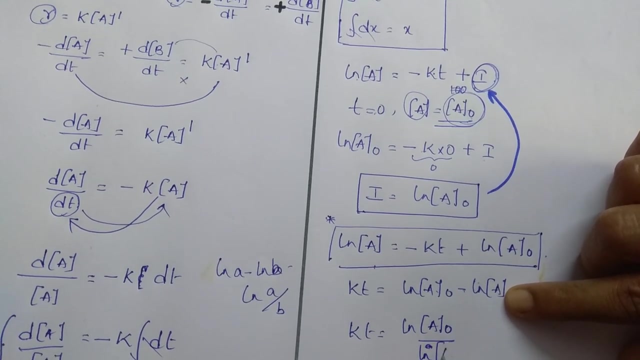 ln of a by b. it is like ln of a minus ln of b. then it will be ln of a by b. then kt is equal to ln of. this is a naught by a by b, so it will be ln of a. now one more formula. 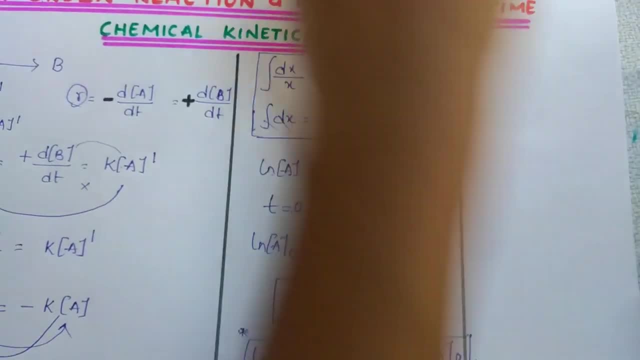 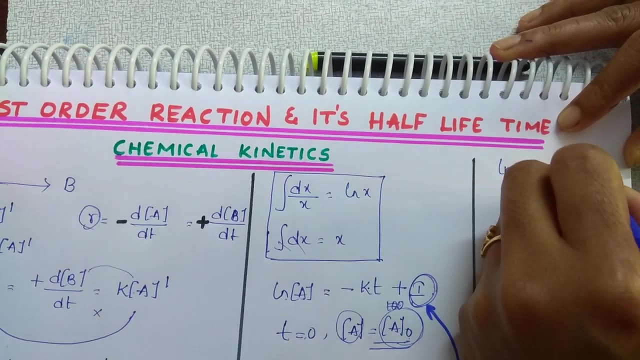 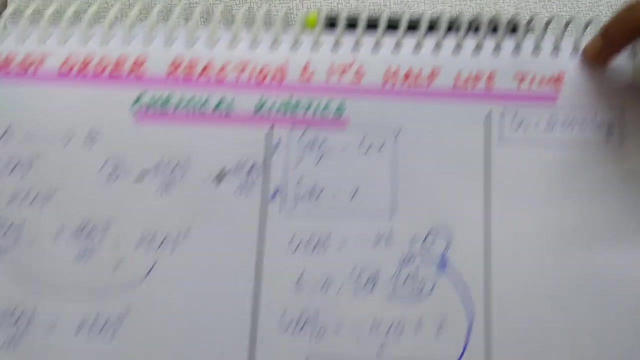 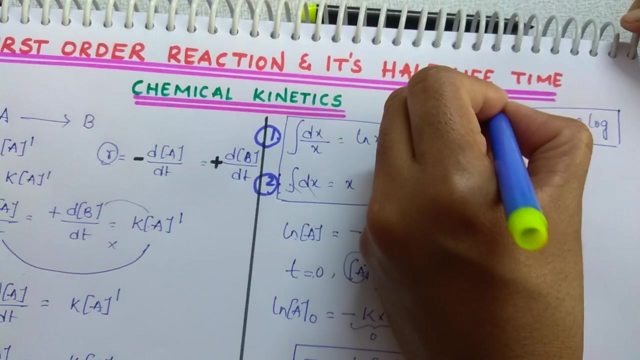 I will tell you ln of how to convert natural logarithm into log is: ln is equal to 2.303 log, so total four formulas. this is formula number one. two: here I used one more formula three, and here I used one more formula four. so kt is equal to here: 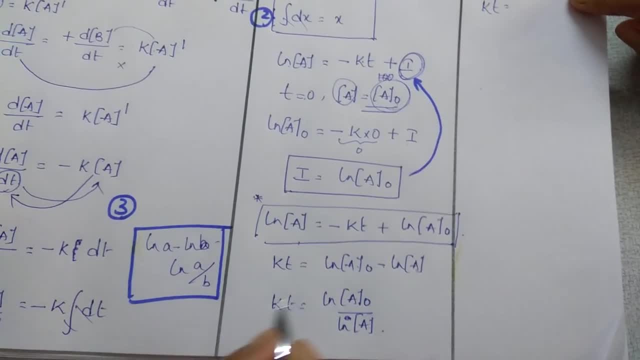 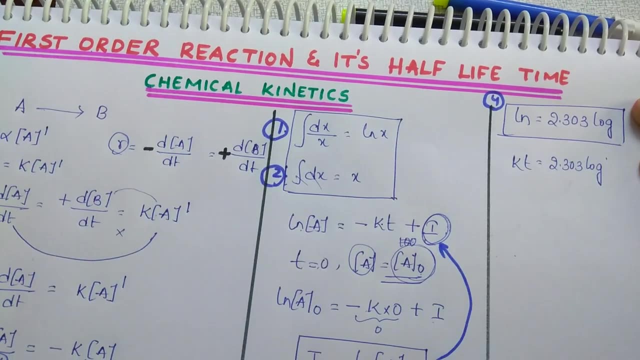 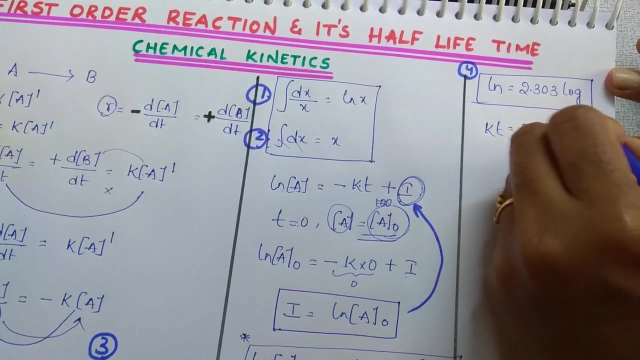 n is equal to this particular formula, and here I will say ln of a minus ln of b by b, ln plus what. I am going to substitute students Here, I am going to substitute 2.303 log. So we get 2.303 log Here. sorry, no ln down, Here no ln. Then log a0 by a. We want rate constant k. 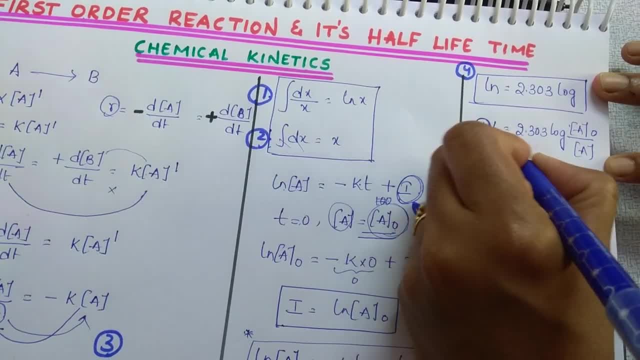 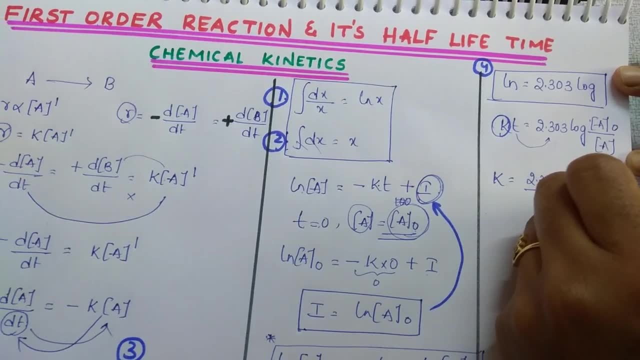 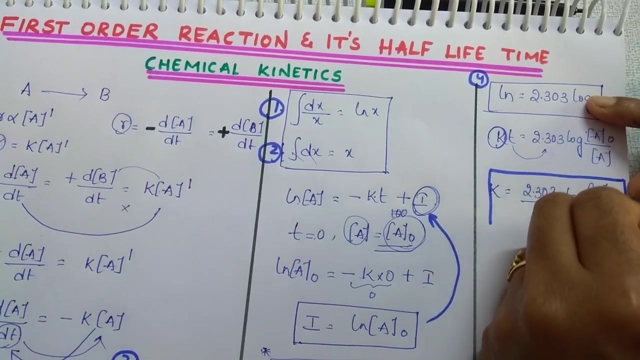 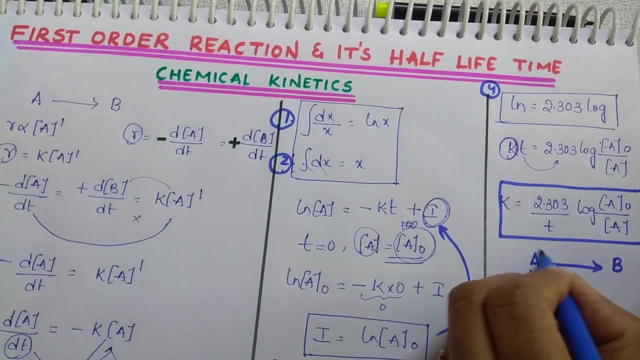 k is equal to Here it is doing multiplication. Move this side, It does division right. So 2.303 by t. log of a0 by a. This is what. This is a rate constant expression for first order reaction. Here a is converted into, a is a reactants and b is a product. So reactants are converting into 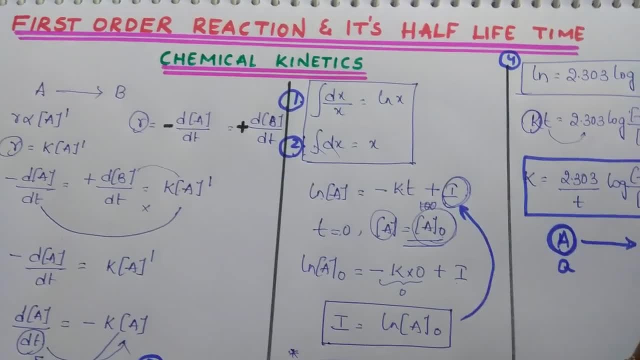 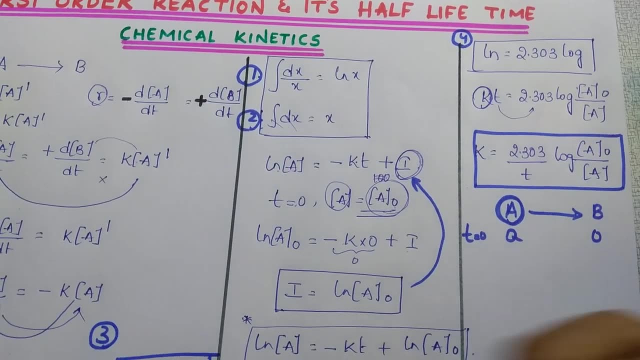 products. Let us take its initial concentration is a, But when reaction is not started, then the concentration: there will be no product. So you can take it as 0. But after some time, t equal to t means after 10 minutes or 15 minutes, what? 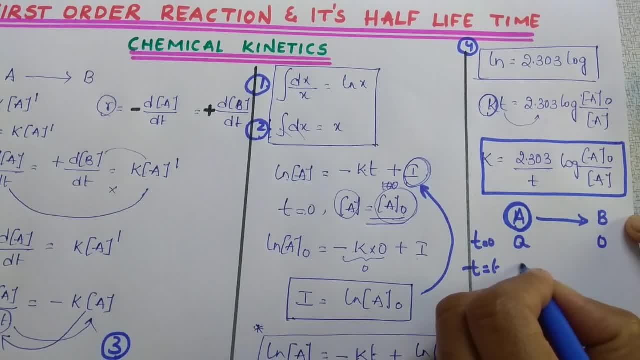 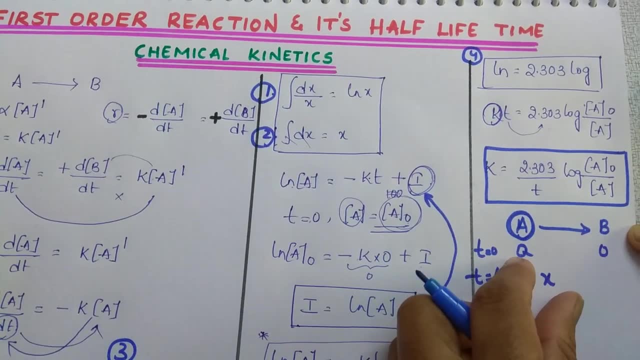 happens, Some amount of a is converted into products. Let us say I will write one more step. X is the amount which is converting from a. That means which x is dissociated from a. Why x is dissociated from a? Because you can. 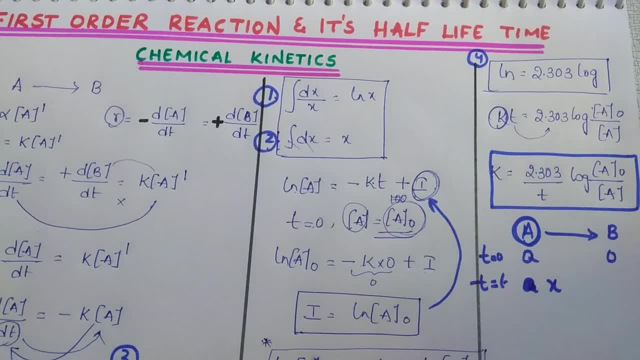 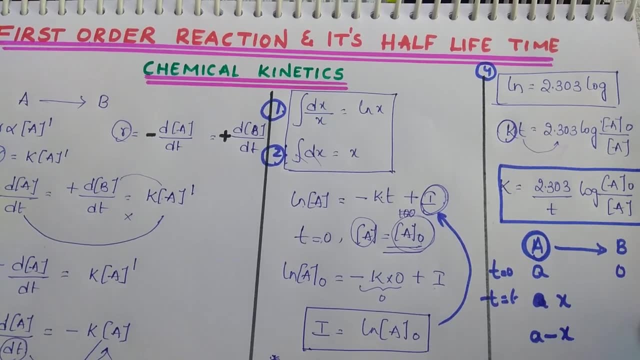 A is converted into product. Let us say this is initially 100 moles, But 25 moles is converted into B. So what you have to do is this: how much is dissociated? you have to subtract from that Then how much it is forming. 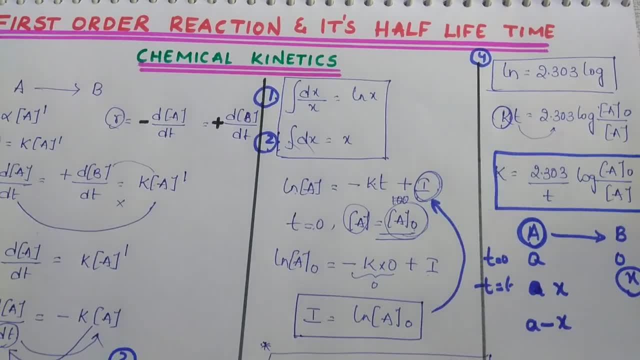 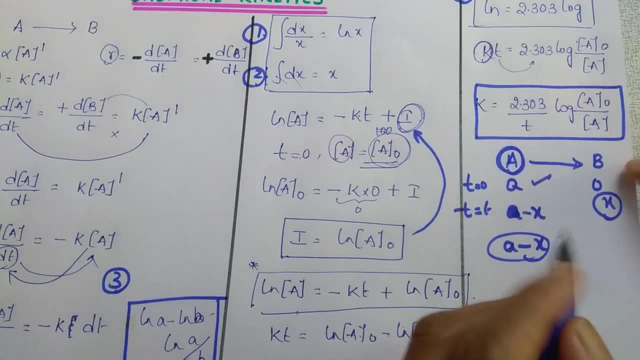 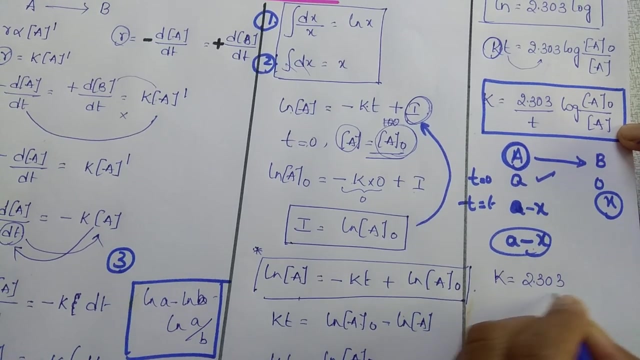 It is forming some X amount. It is forming some X amount. Initially it is initial moles. This is the moles after some time. Then substitute these two expressions in this formula. What you get? K equal to 2.303 by T log of what is A0 students. 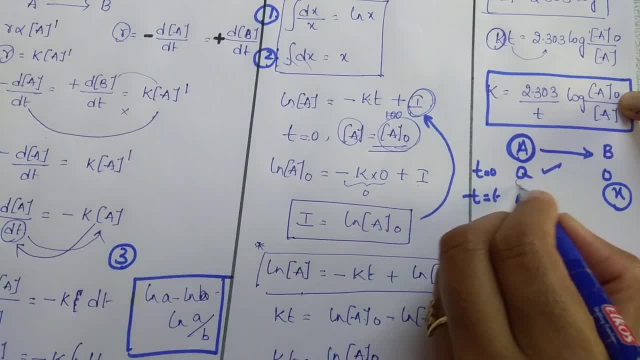 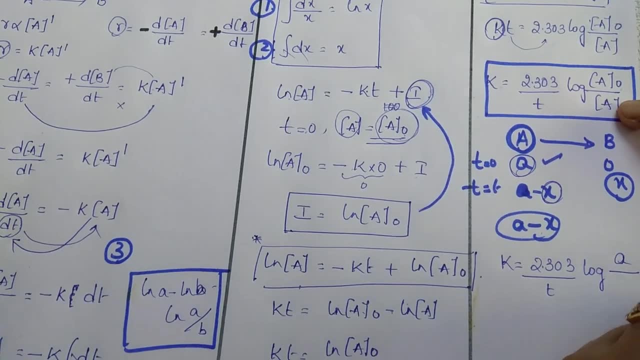 A0 is initial concentration of reactants, So initial concentration we are taking is A And final concentration we are taking A minus X. Some amount is dissociated, So some amount is dissociated. How much amount is dissociated? X amount is dissociated from A. 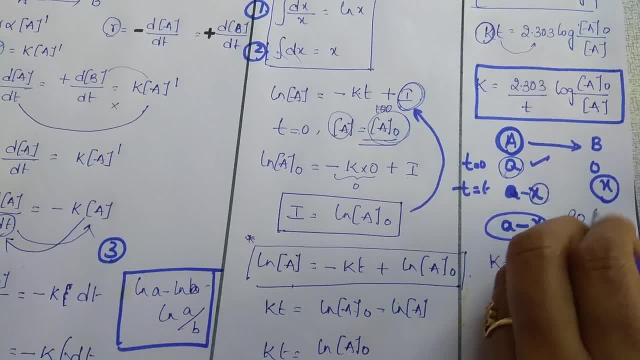 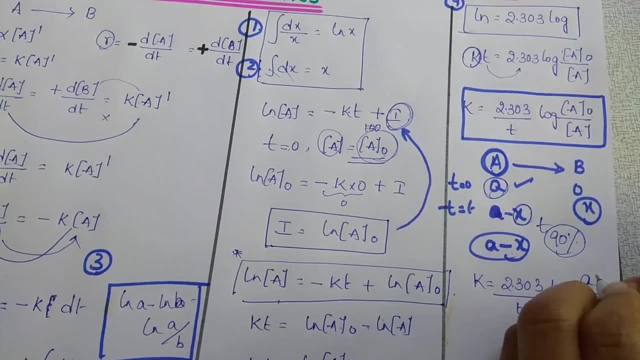 For example, in any reaction they are giving, like 90% of the reactants, Reaction is completed T 90%. What is the meaning of T 90%? A value is initially 100. And A is 100.. From that, 90% of the reactants are consumed. 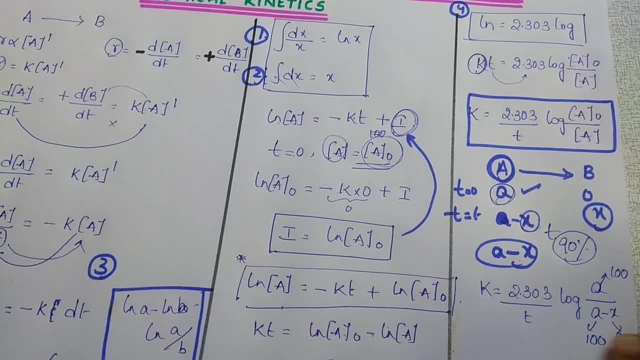 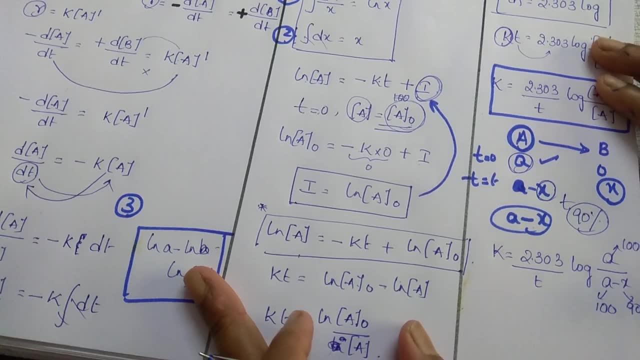 So 90 X value is 90. Then you will get 100 by 10. Then 10 ones are 10, tens are log 10. Log 10 will be 1.. Like that you have to solve the problems Understood. 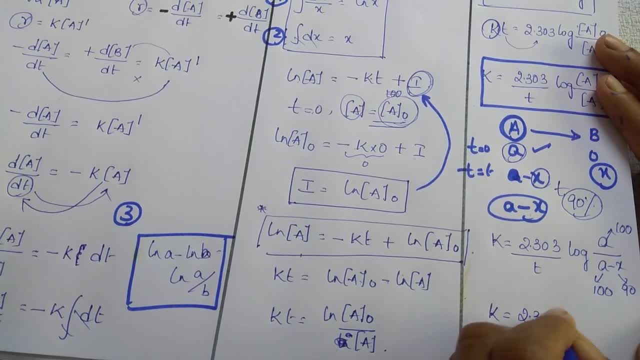 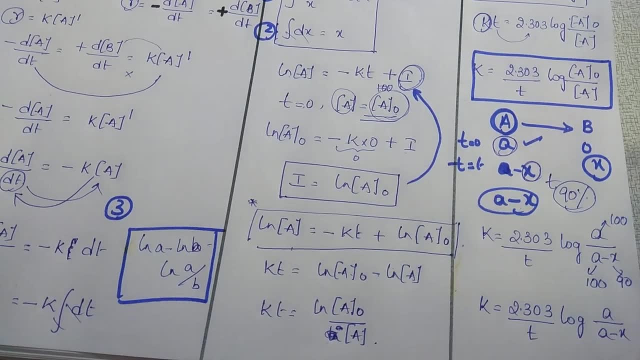 Now this expression you got. What is the expression? K is equal to 2.303.. By T, log of A, by A minus X, This is one more formula. Both are same. Now let us see the graphs for this. 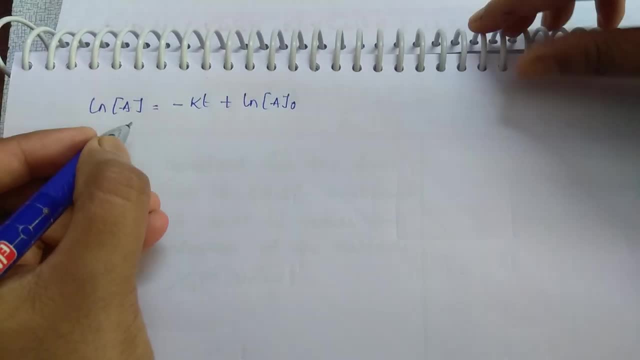 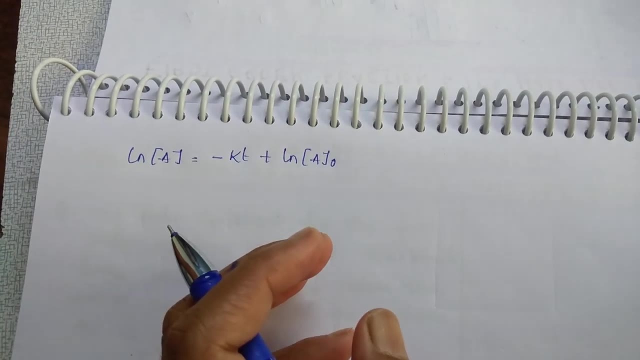 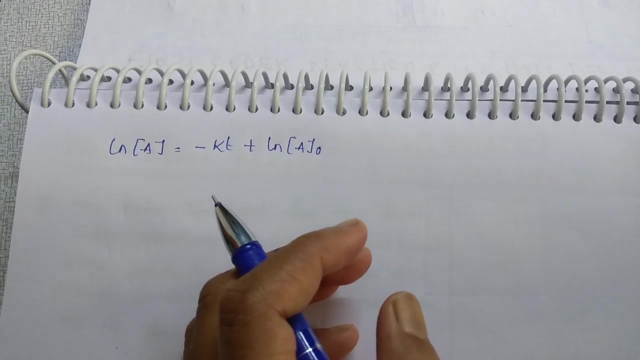 Take this expression- to draw the graphs. Okay, Then what we get here is the use of graph C is They will give the question like: which of the following is the correct graph for first order? reaction Like that: they will ask you. So in those cases, it is very important for you to learn. 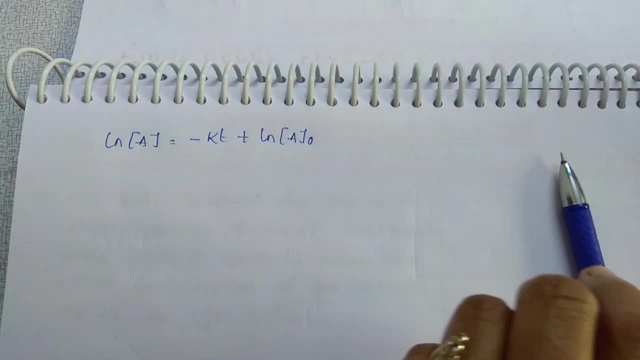 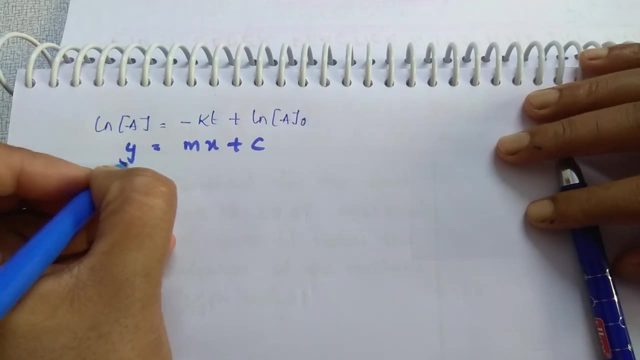 On the graphs. Take, compare this with: Y is equal to MX plus C. Okay, Y is equal to MX plus C. Then this is Y axis On Y axis what you have to take Ln of A On X axis. take time T. 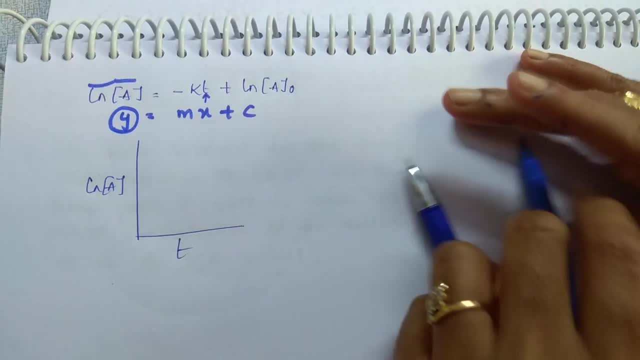 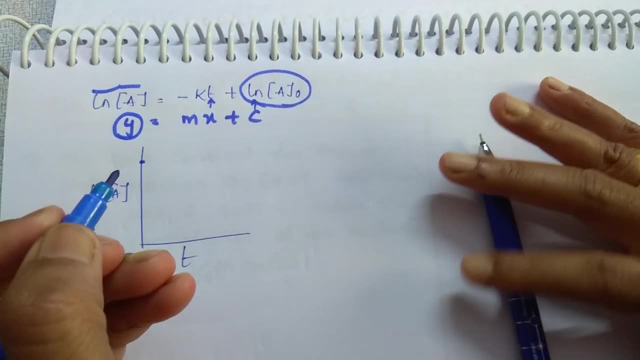 Ln of A On X axis, take time T. Then what is the intercept, students here? C is an intercept, See C means what is the intercept? Ln of A, What do you? What is the meaning of intercept? Simply to say the line or the curve which cuts the Y axis. 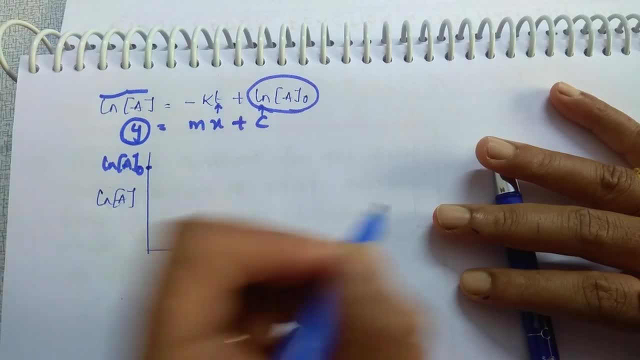 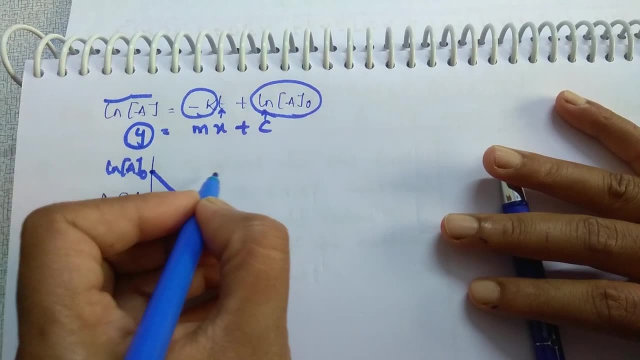 So here let us take here Ln of A0.. And here M. M is a slope. Slope is what Minus K, Negative slope. So it comes down. Graph is like this: Slope is equal to minus K. 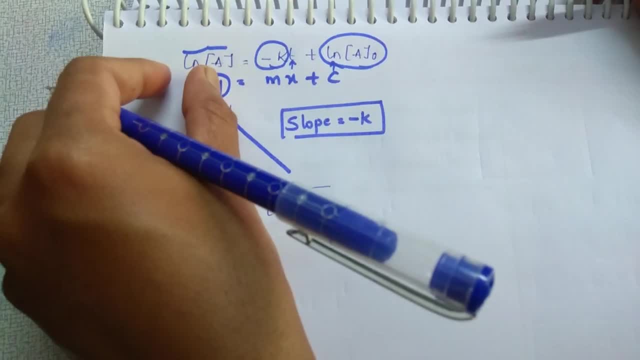 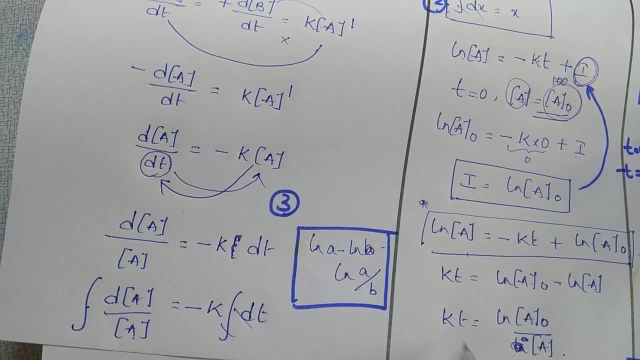 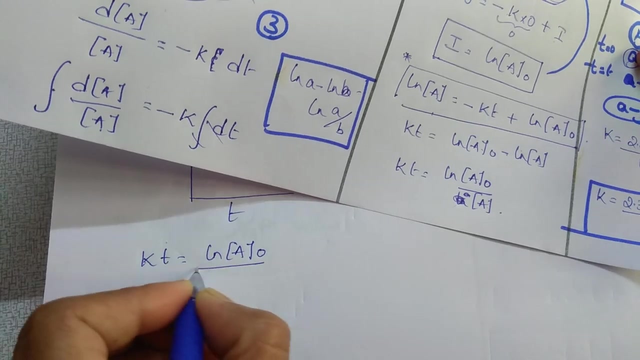 From this expression only. what I do is I move KT this side and Ln this side. Then what we get, or otherwise, directly Already I did so I can take from this directly: KT is equal to this expression. I am taking Ln of A0 by A correct. 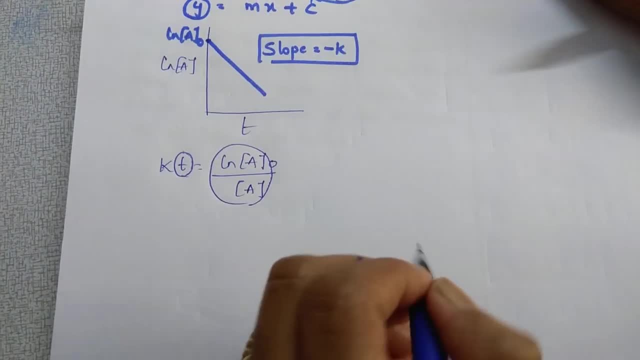 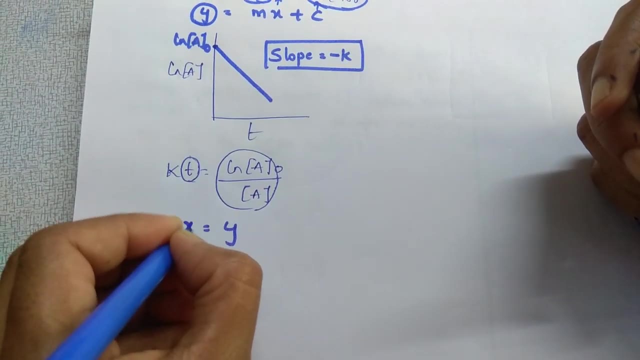 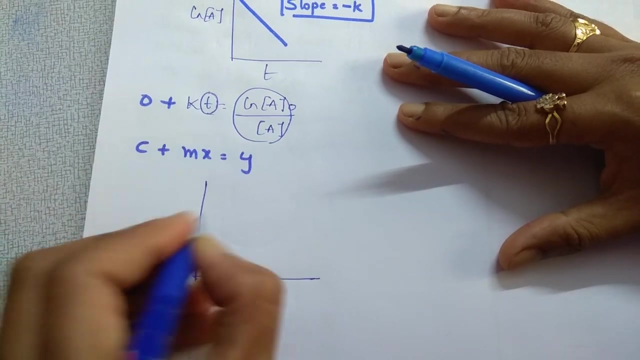 Now draw the graph between Ln of A0 and T. Here there is no intercept. It is like Y is equal to this is Y. We are taking this on Y, axis MX, and here there is no slope. no slope, which means that if you draw the graph on Y, 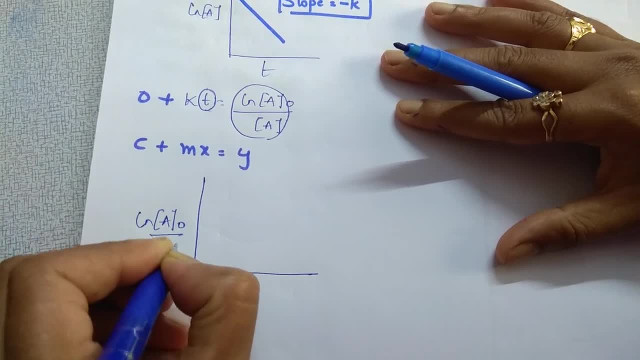 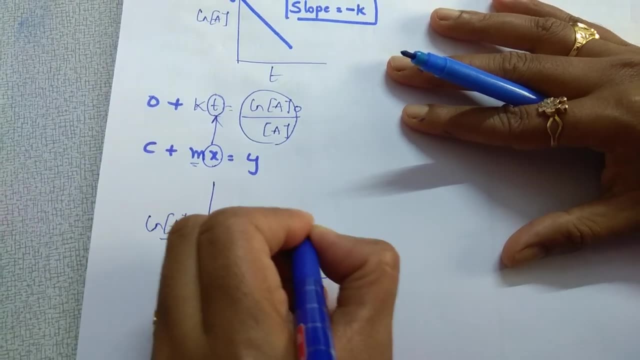 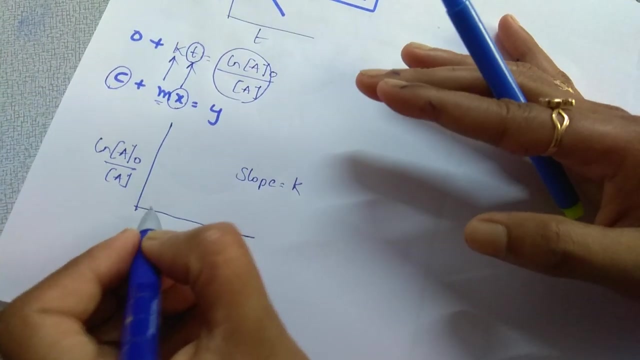 Y axis you are taking Ln of A0 by A and on X axis what you are taking students time you are taking and slope here is positive slope. slope is what K, slope is K and here there is no intercept. So line passes through origin like this, and because Y slope is and that is, slope is positive. 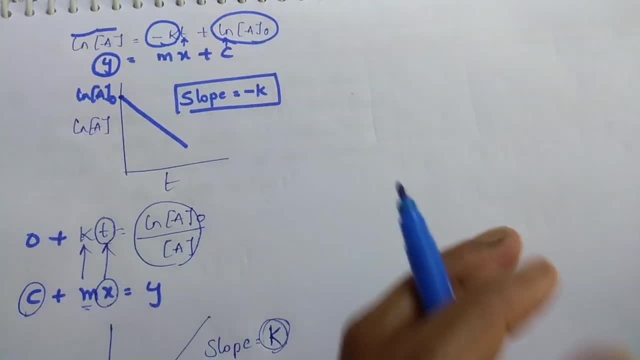 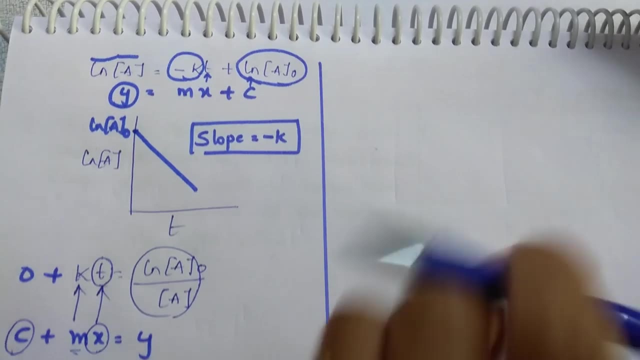 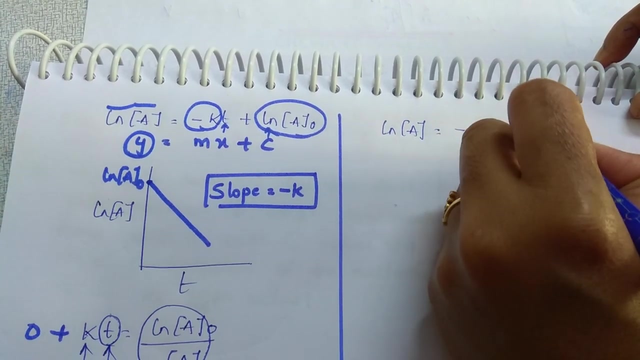 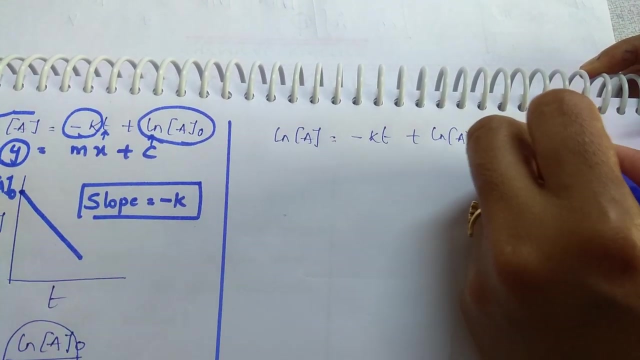 slope. take this expression. So line passes through origin like this: Ln of A is equal to this only. again, I am taking minus KT plus Ln of A0.. In this how to convert this into log, Ln is equal to 2.303. log substitute in place of. 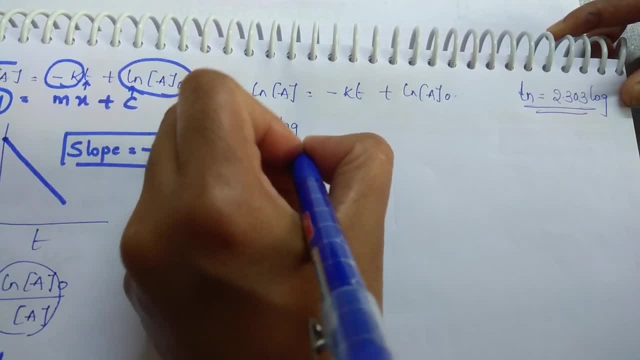 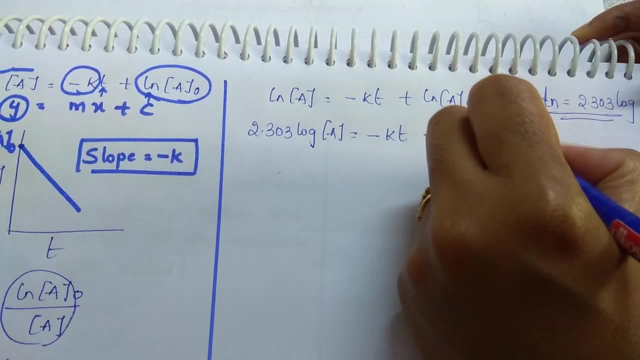 Ln 2.303 log. So 2.303 log of A minus KT. So this is Ln of A0. Plus 2.303 log of A0. just what we did. we substituted 2.303 log in place of Ln divide on both the. 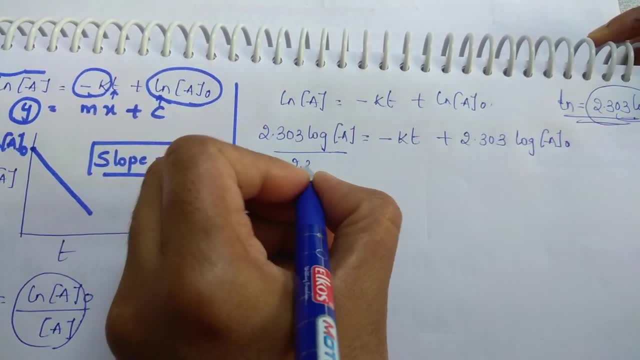 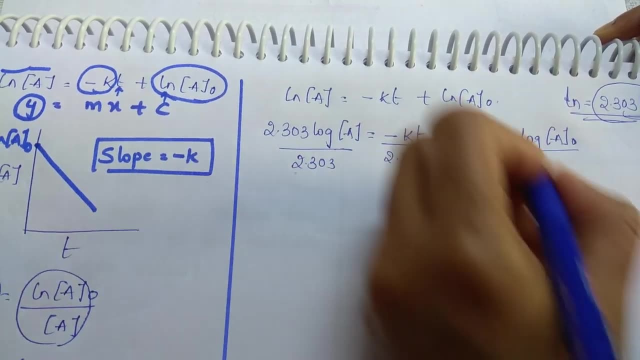 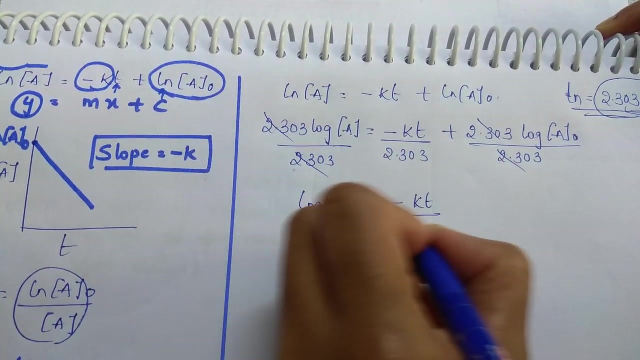 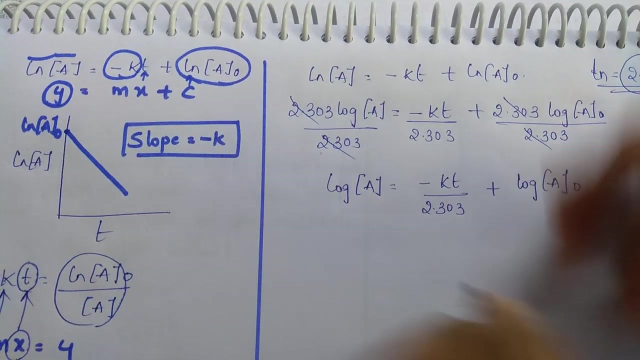 sides with what? 2.303. same step again here. only I am doing: when you are doing, do it in separate step while practicing in exam. it is not required. then you get log of A is equal to minus KT divided by 2.303.. Now draw the graph for this. this is: Y is equal to Mx plus C. compare this with straight. 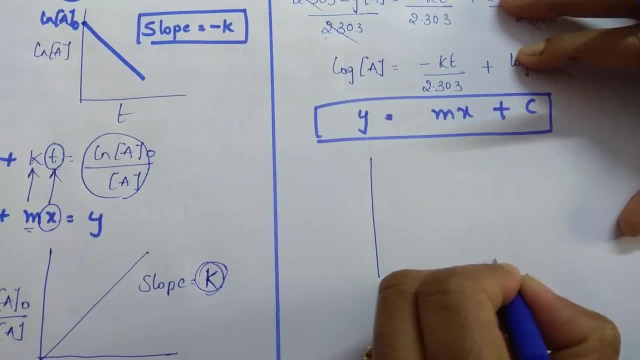 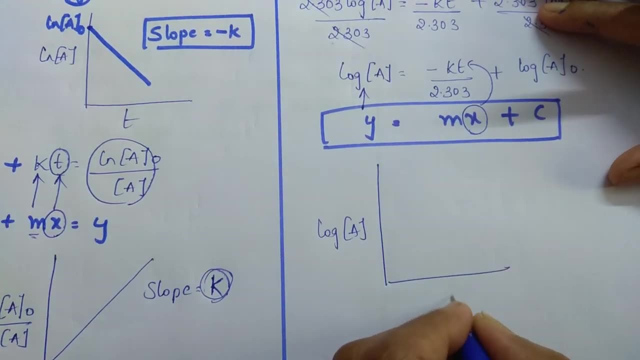 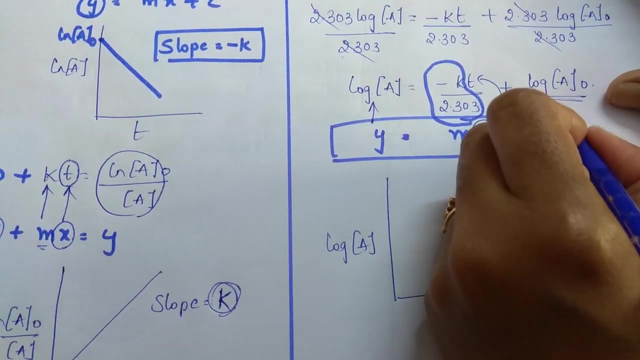 line equation, again on Y axis, what you have to take, students, tell me on Y axis, take log of A on X axis what you have to take, take time then. what is the slope over here? minus K by 2.303, what is the intercept? C is in log A0.. 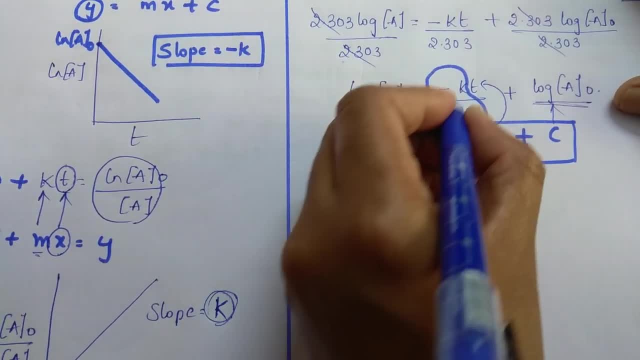 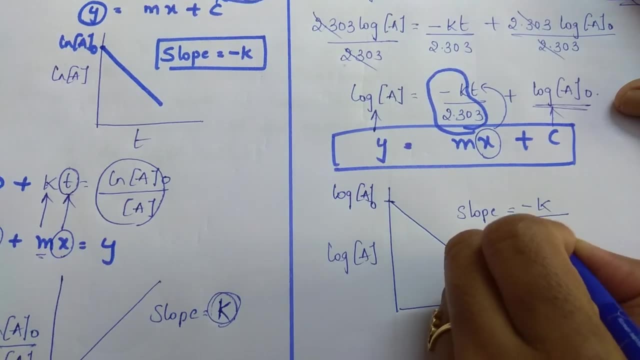 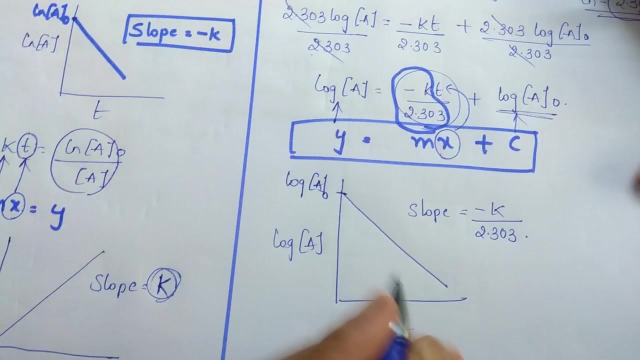 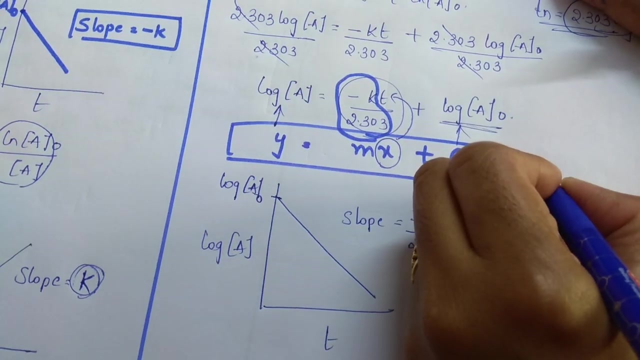 Log A0 is an intercept and here negative slope. so slope comes down like this: slope is equal to minus K by 2.303.. Clear and again, you can move this also: KT this side and Ln A this side. then what you get, tell me: KT by 2.303 this side, you move, and this term you move this side. then log of A0. 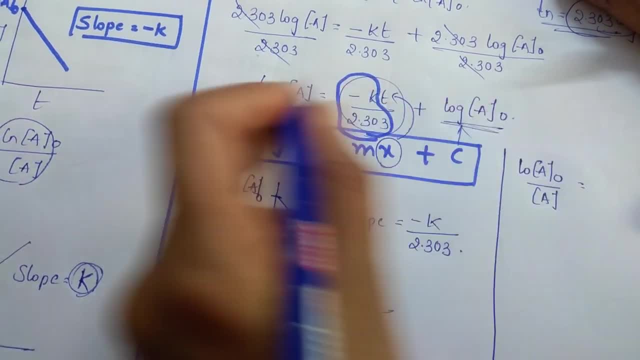 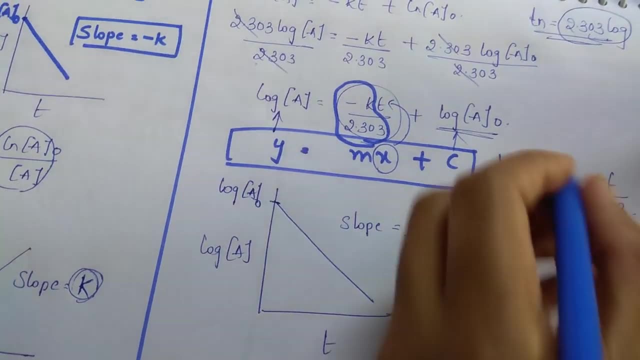 by A Right, Because it is like log of A minus log of B. Then it will be log of A by B, KT by 2.303.. Then compare this with: Y is equal to MX plus C. There is no intercept. 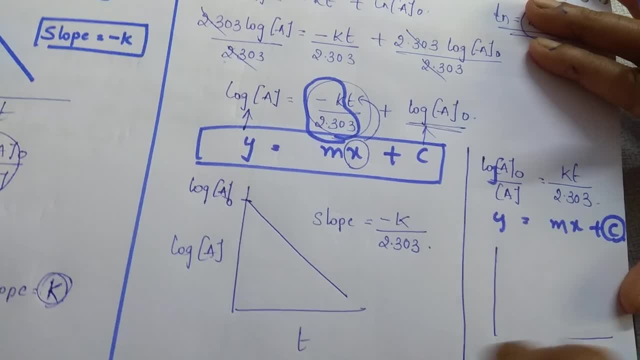 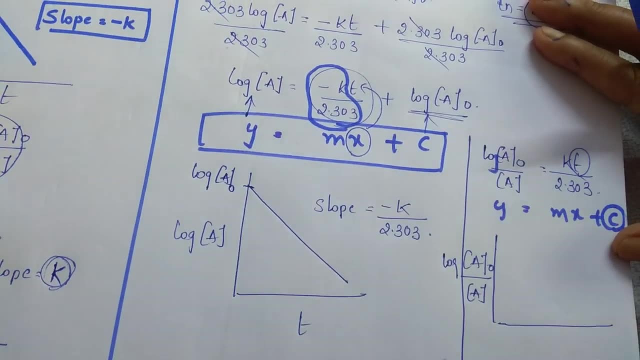 Intercept is 0.. No intercept. So you get on Y axis what you have to take. students, tell me Log of A naught by A And on X axis what we are taking. Time T And what is the slope? No intercept. 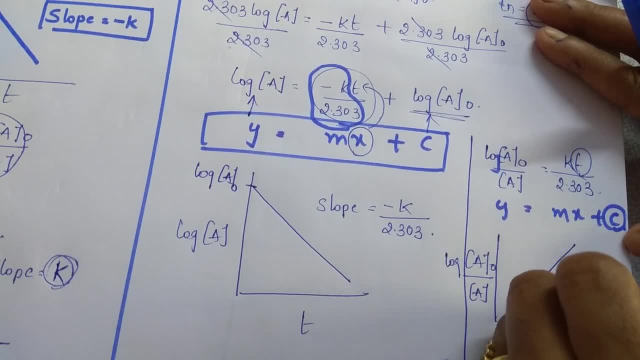 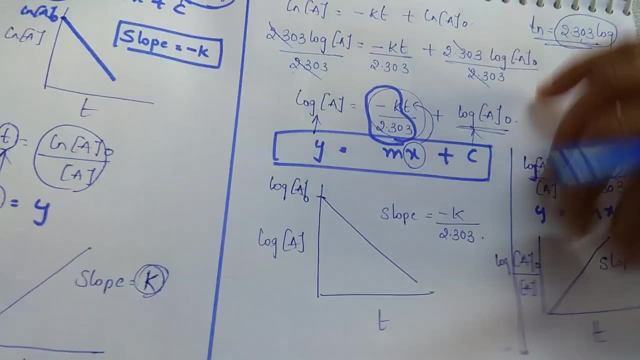 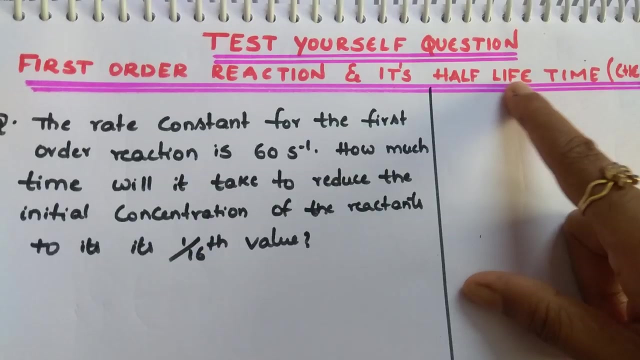 So line passes through origin like this. And what is the slope? Slope is equal to K by 2.303.. Let us see half-life time. Try this question and comment me your answer. I am going to do half-life time and solution to this problem in next video. test yourself solution. 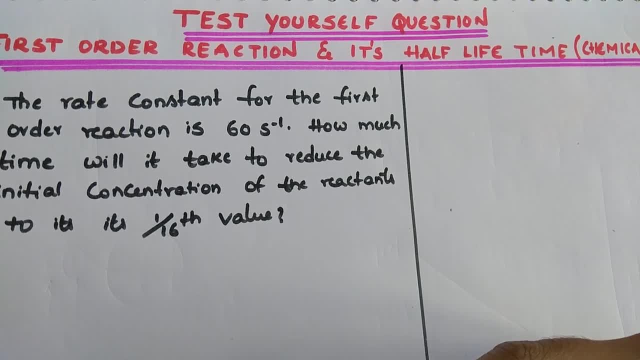 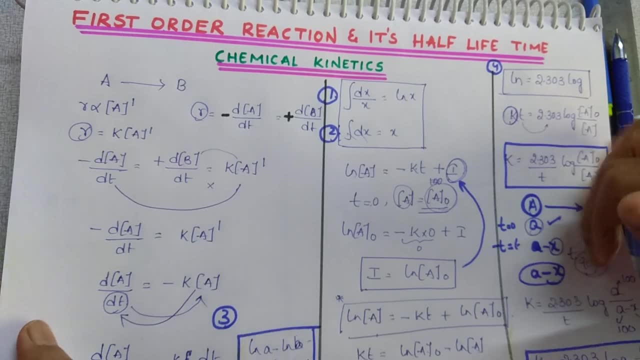 My name is Komali. Thank you so much for watching. I hope you like this. Please give a big thumbs up.